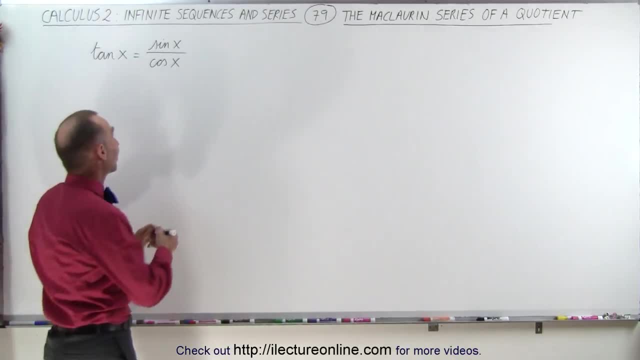 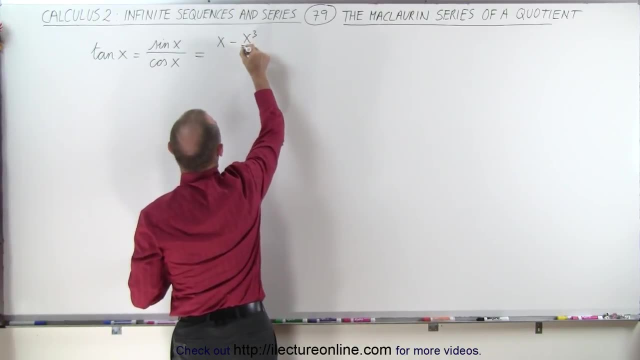 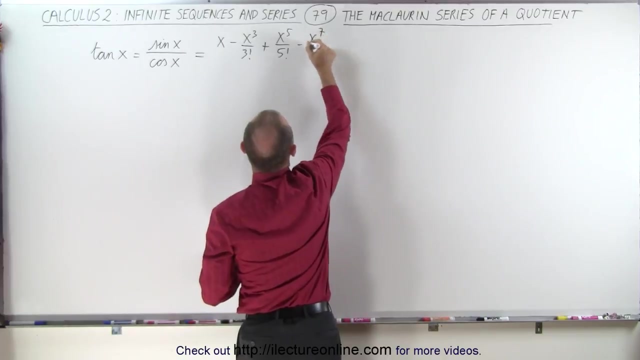 Hmm, what does that look like? Well, let's take a look. This is equal to in the numerator. we end up with x minus x cubed over 3 factorial, plus x to the 5th over 5 factorial, minus x to the 7th over 7 factorial, and so forth. 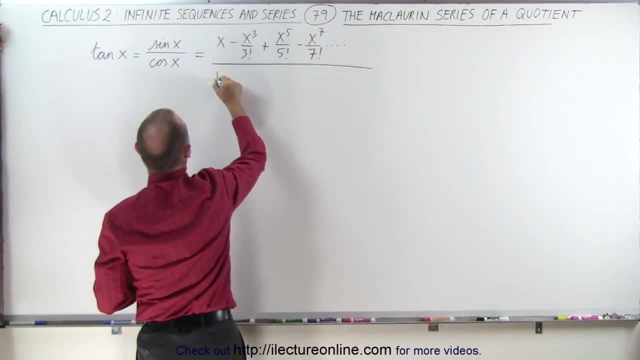 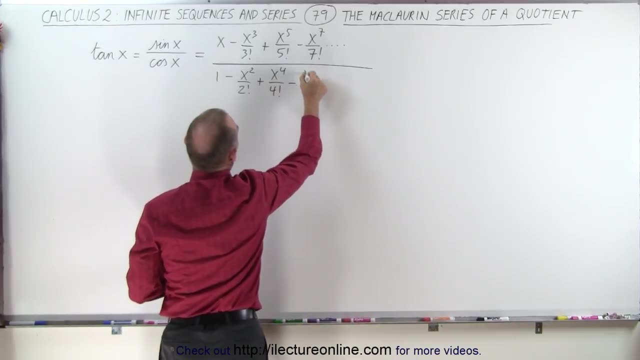 And we're going to divide that by the cosine of x, which is 1 minus x squared over 2 factorial, plus x to the 4th over 4 factorial, Minus x to the 6th over 6 factorial, and so forth. 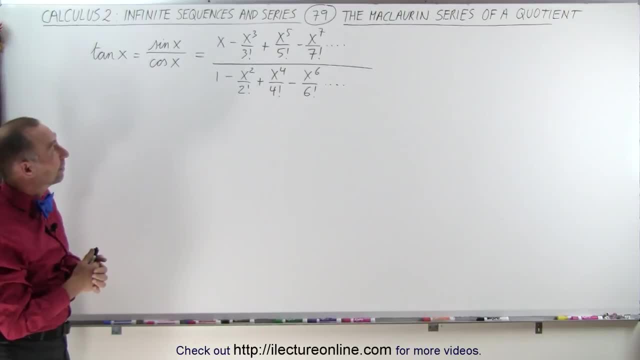 Now again trying to divide one infinite sum by another infinite sum. that seems kind of crazy. And yes, it would be if you try to do it for that many terms. But if we limit the number of terms it is actually doable. 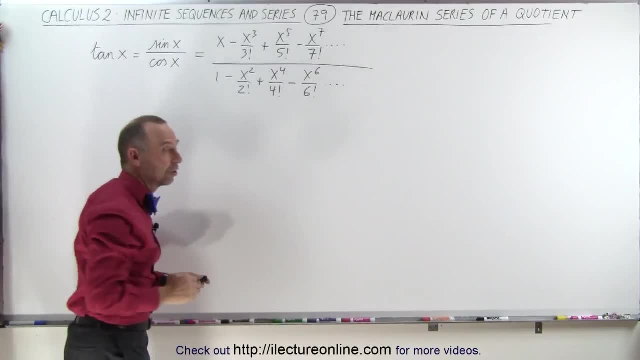 And perhaps we should only limit ourselves to the first three terms. So let's go ahead and do that. Let's divide the first three terms of the sine of x By the first three terms of the cosine of x and see what we end up with. 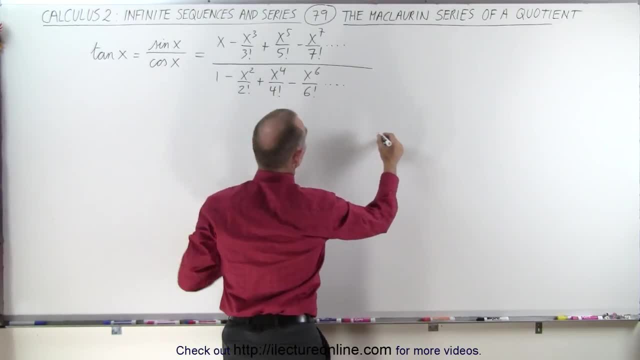 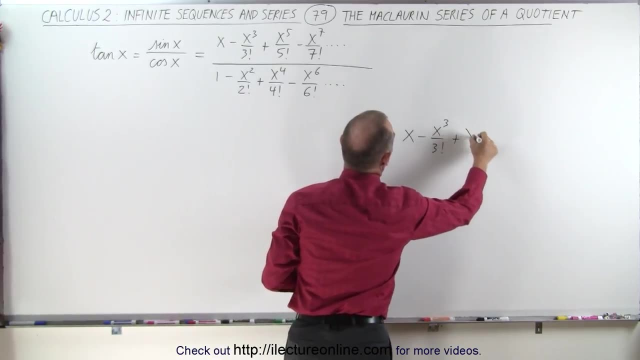 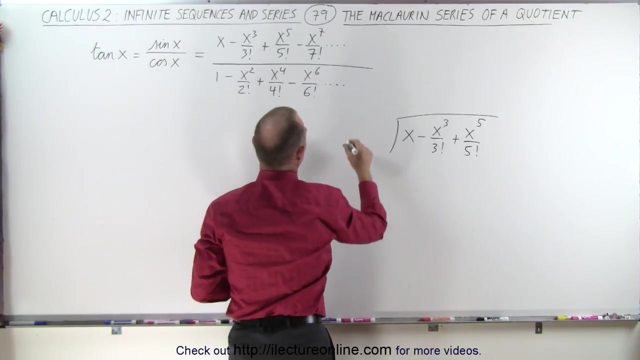 So here we can say that we're going to divide into the numerator. The numerator is x minus x cubed over 3 factorial, plus x to the 5th over 5 factorial, And we're going to divide into that the first three terms here, which is 1 minus x squared over 2 factorial, plus x to the 4th over 4 factorial. 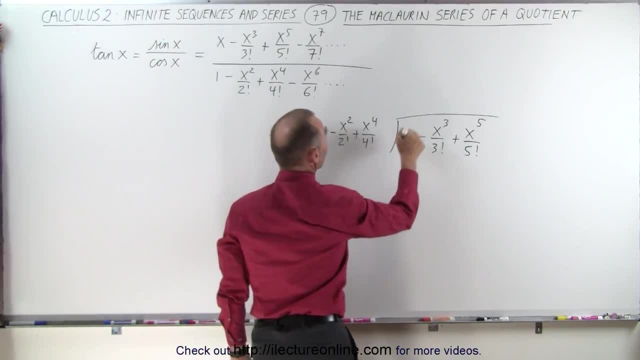 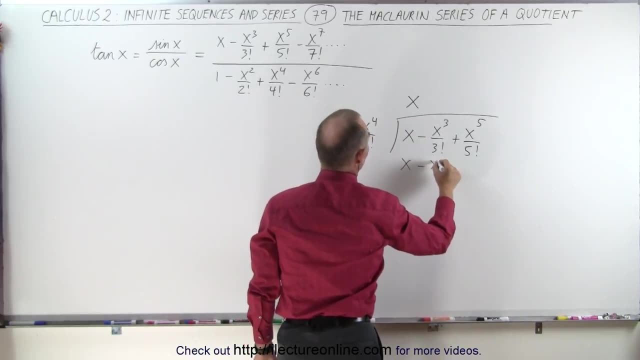 So let's go ahead and do that and see what we get. Well, 1 goes into x, x times goes to x times. 1 is x, x times minus x. squared gives us minus x cubed over 2 factorial And x times. this gives us plus x to the 5th over 4 factorial. 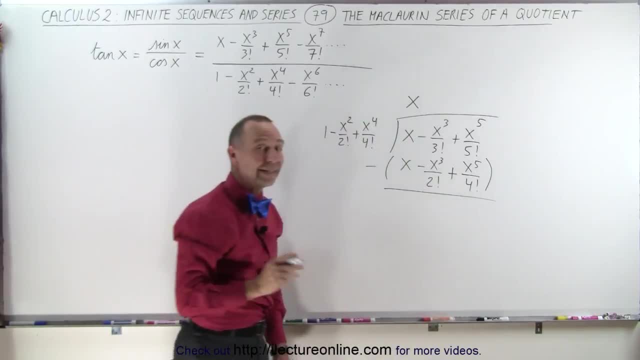 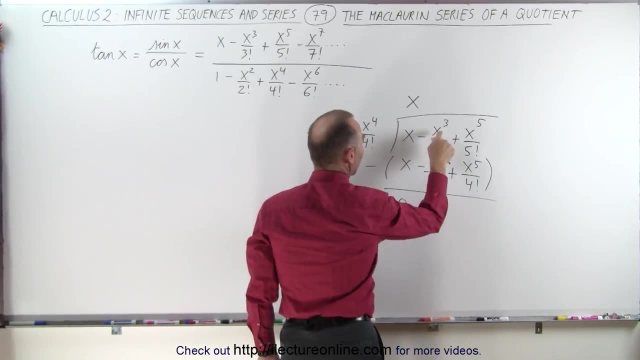 Now we can subtract. Luckily the exponents and the x's do line up. So here we have x minus x, which is 0. And x cubed over 3 factorial minus x cubed over 2 factorial. But it's a minus times a minus, so this is actually a plus. 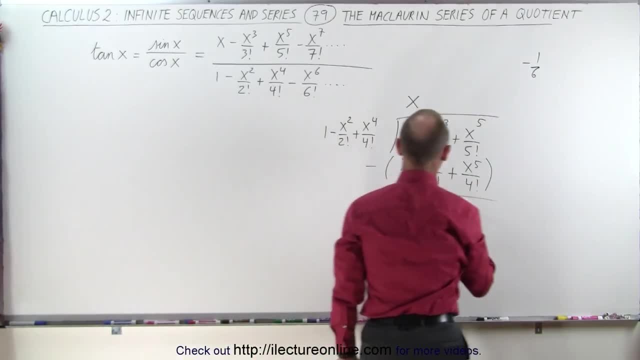 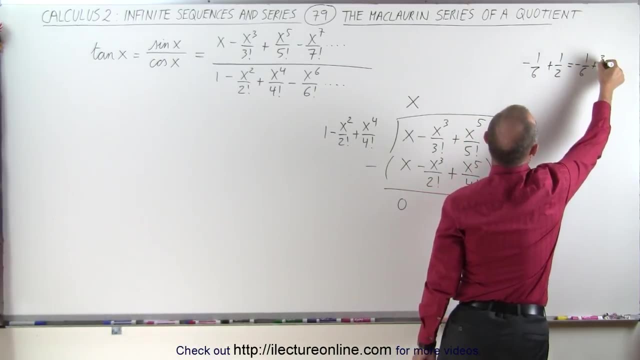 So we end up with a minus 1 sixth in the denominator plus 1 over 2.. And that would be equal to minus 1 sixth, plus 3 sixth, which is equal to 2 sixth, which is equal to 1 third. 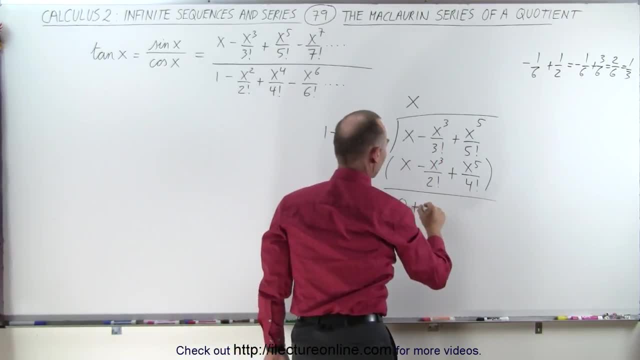 So when we subtract this from that, we end up with plus 1 third, So that's x cubed. And then here we're going to subtract this from that, So we end up with a 1 over 120.. That's 5 factorial. 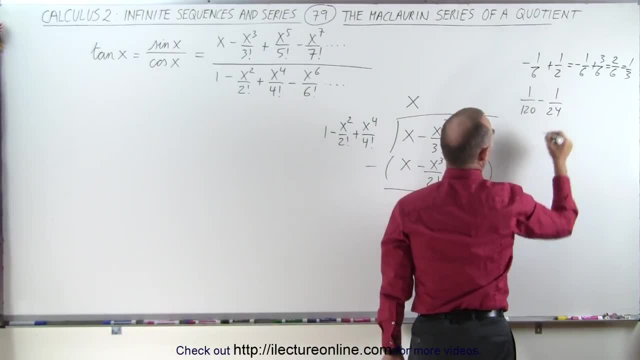 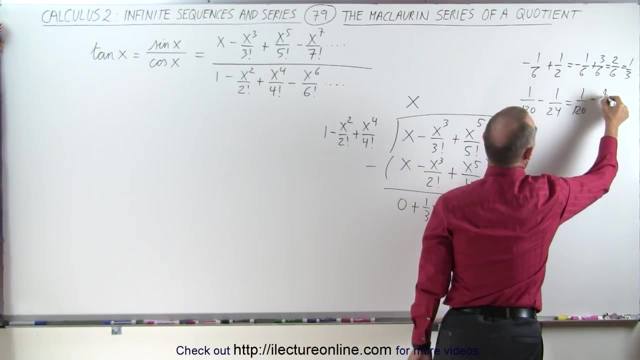 Subtract from that 1 over 4 factorial, which is 24.. Common denominator is 120.. So 120 minus 1 over, not 1, but 5 over 120, which is minus 4 over 120, which is minus 1 over 30.. 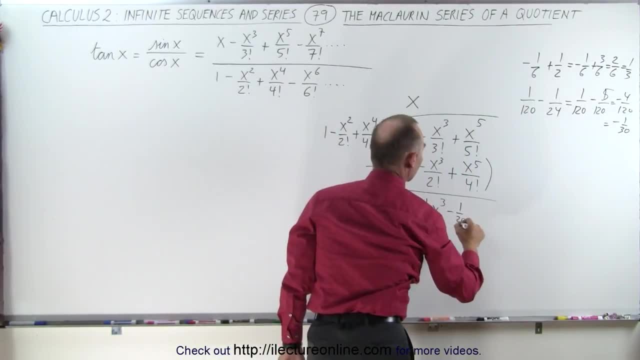 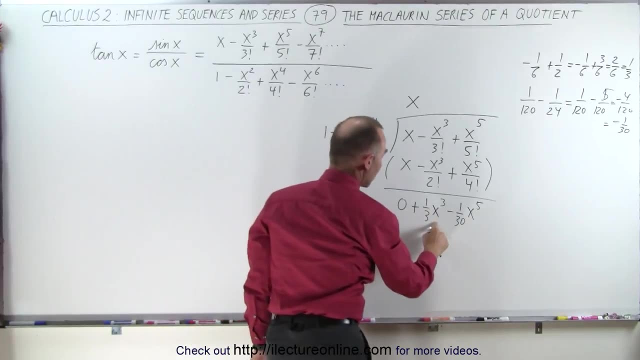 So the result: here: we get Minus 1 over 30th x to the 5th power. So we're not done yet. Now we're going to divide 1 into here, which is plus 1 third x cubed. 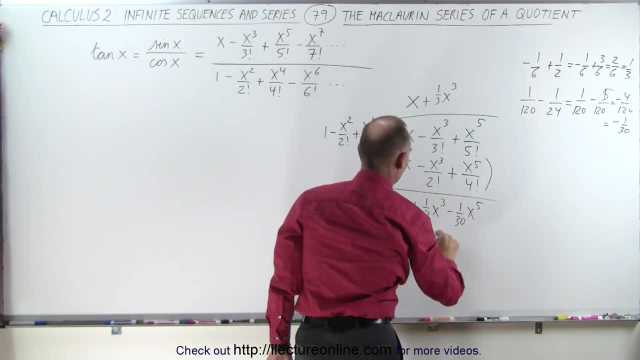 Because this times this gives us 1 third x cubed, And this times the second term will give us 1 over 6. So minus 1 over 6 times x to the 5th, And we're not going to multiply this times this. 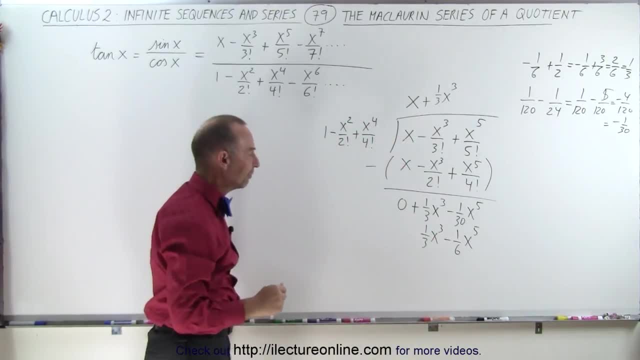 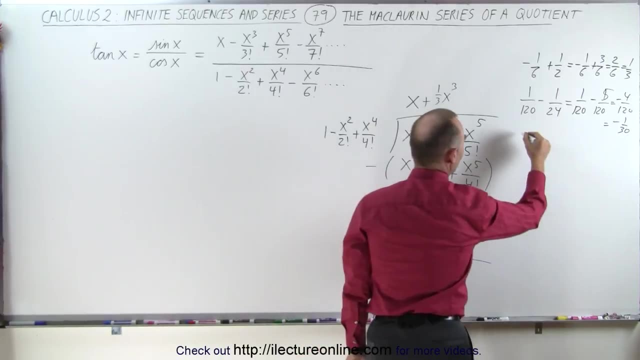 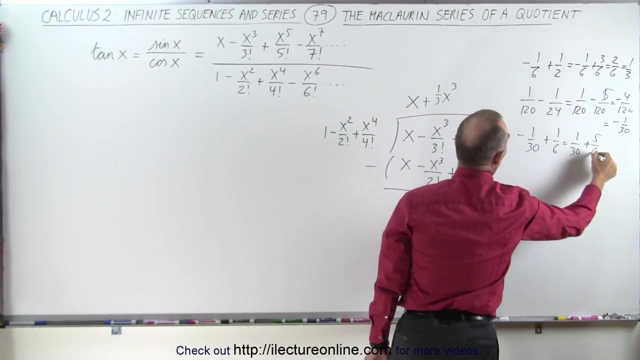 Because we're going to ignore any terms that have a greater exponent than 5.. So when we subtract this from that, we get 0. And subtracting a negative becomes a positive. So we have minus 1 over 30 plus 1 over 6, which is minus 1 over 30 plus 5 over 6,. 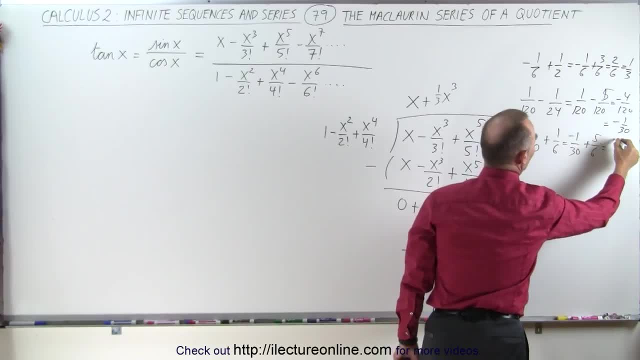 which is equal to that should be minus. so that gives us 4 over 30.. So that gives us 4 over 30,, which is 2 over 15.. So plus 2 over 15, x to the 5th. 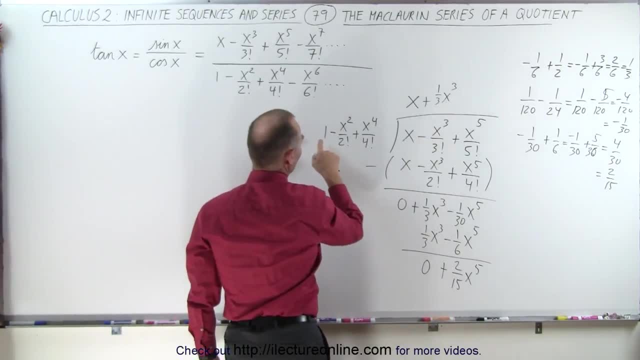 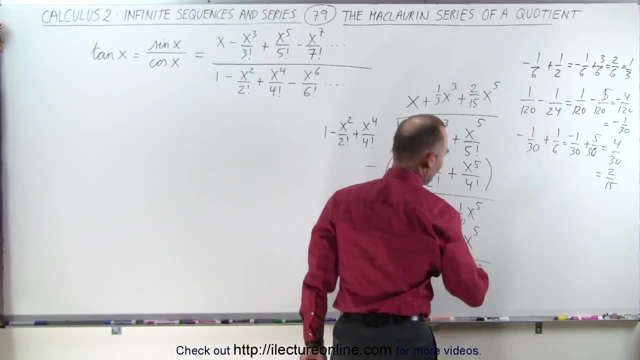 And then for the last term here in the quotient we say 1 goes into here, Plus 2 over 15 x to the 5th times, And then we don't have to worry about the rest. So here we have the first three terms of the quotient.